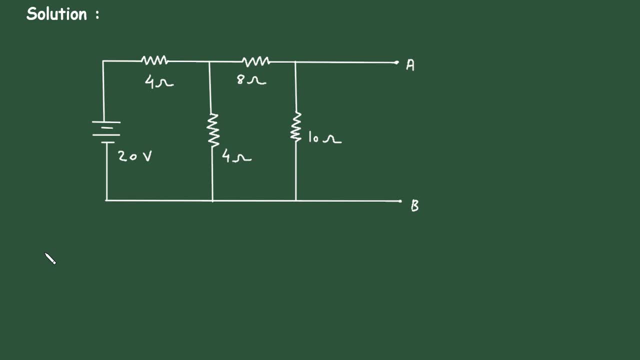 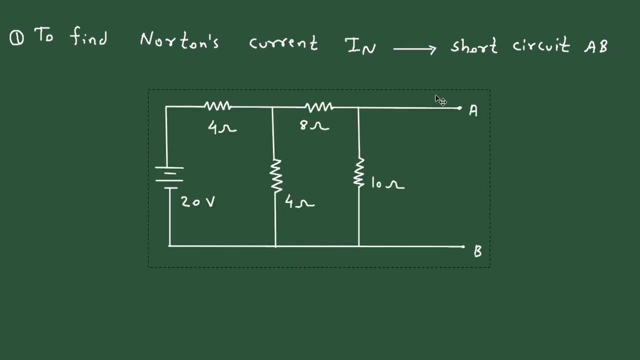 current. So to find Norton's current, to find Norton's current I? n, we have to short circuit terminal a b. This will be our step number one: short circuit, short circuit terminal a b Now here. if we short circuit terminal a b, then this will be our current I? n, Now here. 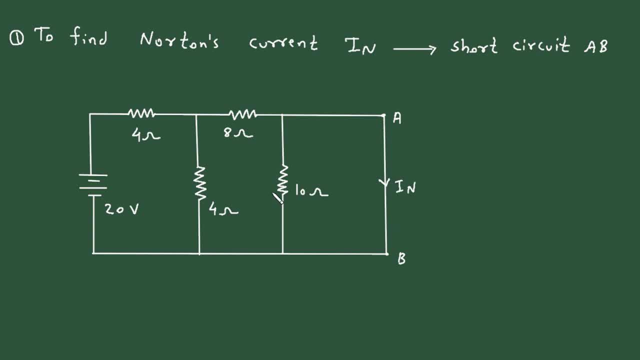 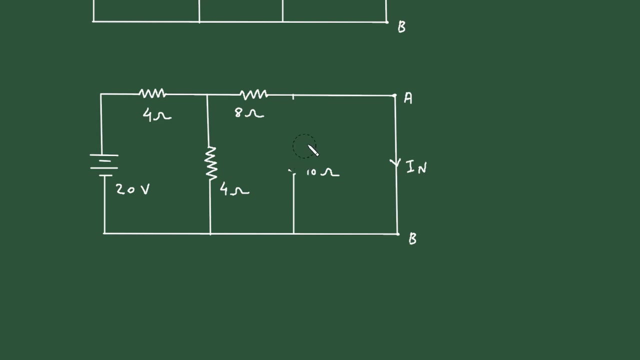 we can see if we short circuit terminal a, b, that time this 10 ohm resistor will be zero. So again, we can copy this circuit and we can remove this 10 ohm from here. Now we can find true value passed through. Let me solve an experiment or I will have. 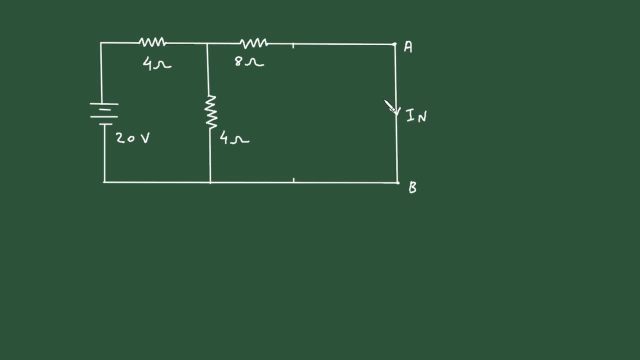 some CAS test, You can find the value of this current I n, which is the current, flowing through this 8 ohm. Now you can find the value of this current I n, which is the current flowing through the 8 ohm, with current division rule. if I can find the value of current Darby To do this. 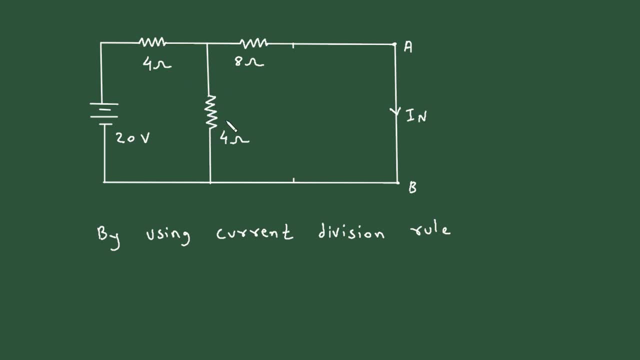 first of all, we have to find the value of this current. let's say this current is current I. now here we can see this: 8 ohm and 4 ohm are connected in parallel, so the resistance value will be. or we can directly find the value of current I. I is equal to V by R, the 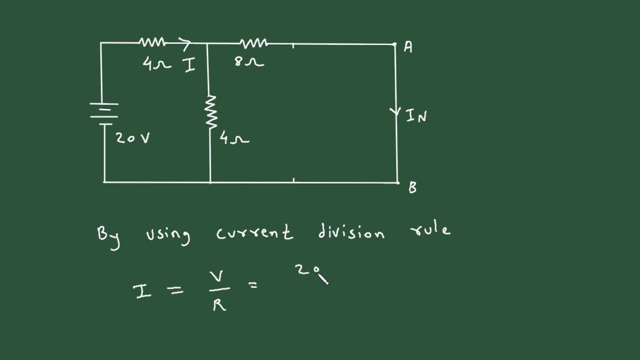 value of voltage is 20, so 20 divided by the value of resistance R, so resistance R will be total equivalent resistance. it will be this: 4 ohm plus, and these are in parallel. so it will be 4 into 8 divided by 4 plus 8. so this will be 20 divided by. 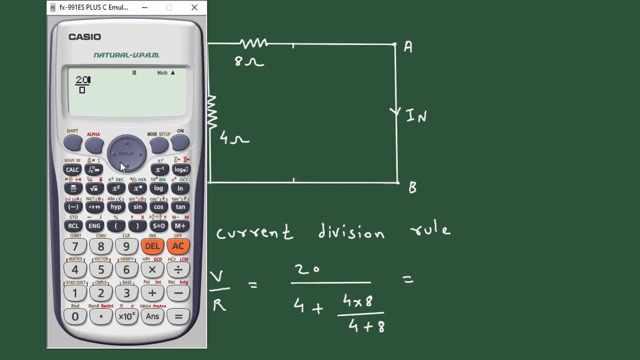 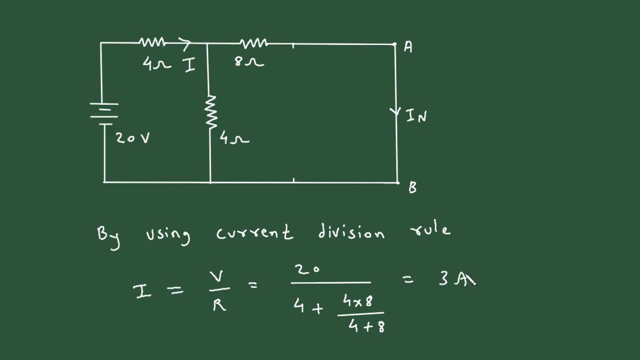 20: 20 divided by 4 plus 4 into 8 divided by 4 plus 8. so it is 3 ampere. the value of this current is 3 ampere. now we can use current division rule. so here we have to write this: 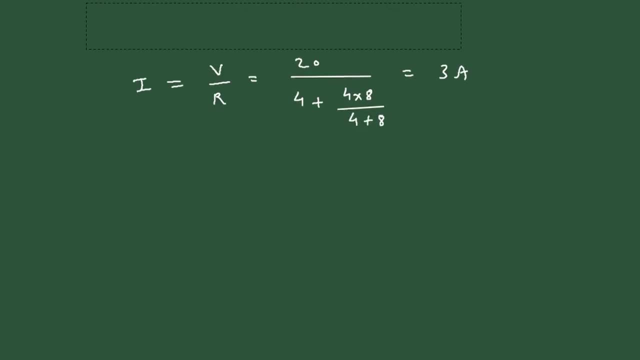 current division rule here now. current division rule I I n is equal to this current, that is I. current I and current I is 3 ampere, so 3 multiplied by opposite branch resistance is 4 ohm, so 4 divided by 4 plus 4 plus 8. so this will: 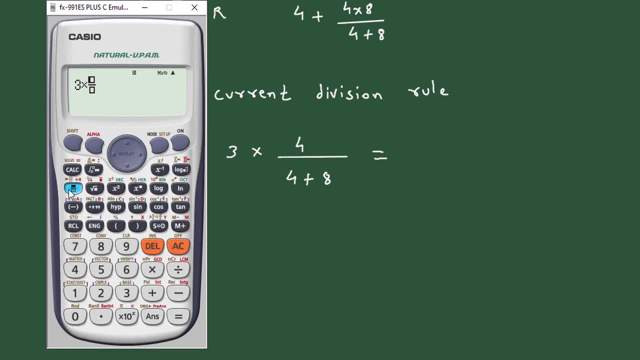 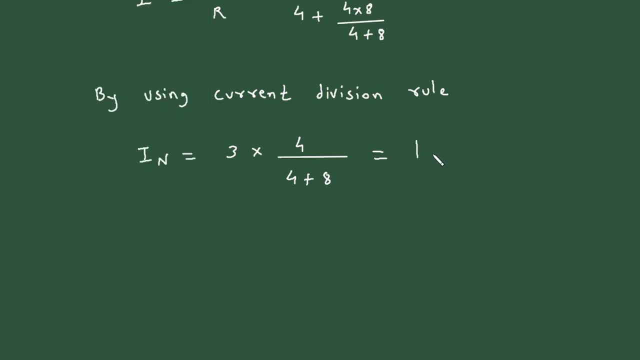 be 3 into 4 divided by 4 plus 8, so it is 1 ampere. the value of Norton's current is 1 ampere. I n is equal to 1 ampere now. next we have to find Norton's resistance. step number 2: find Norton's resistance now. to find Norton's resistance R n, we have to: 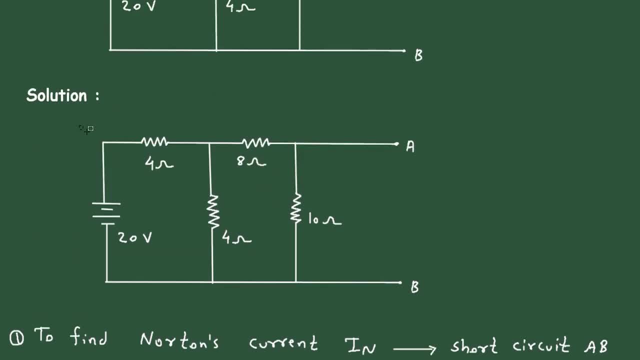 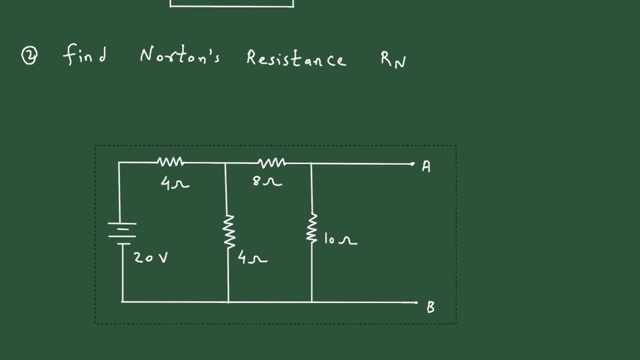 turn off all the independent sources. so here this is our circuit. now here we can write to find R n: turn off all independent sources. now, here there is only one independent source and that is a this voltage source. so when we turn off the independent voltage source, that 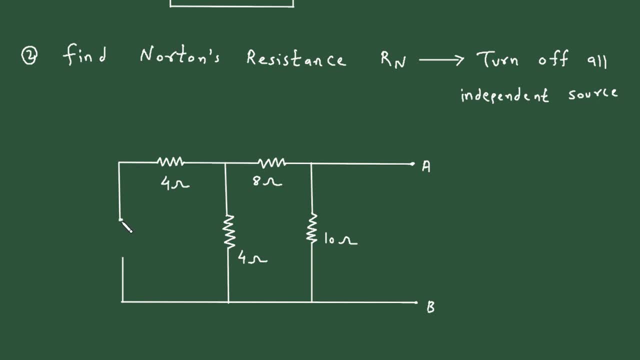 time it will be short circuit. we have to replace this by its internal resistance, so it will be short circuited, and this will be our resistance R n. so this will be our resistance R n. now, here we can see. this 4 ohm and this 4 ohm are connected in parallel. now we will simplify. 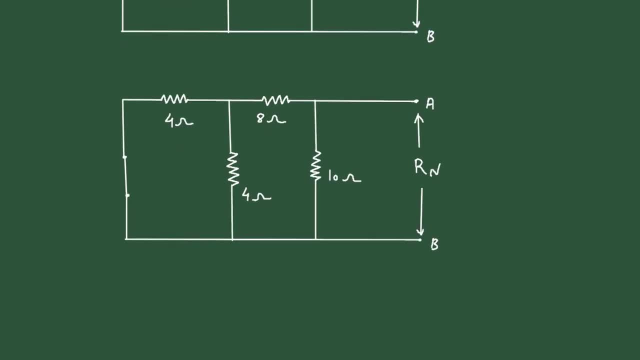 this circuit, so this 4 ohm and this 4 ohm connected in parallel, so this will be of 2 ohm. when two resistance of same value are connected in parallel, that time we have to write. its parallel equivalent will be half of it, so it will be 2 ohm. now this 2 ohm and 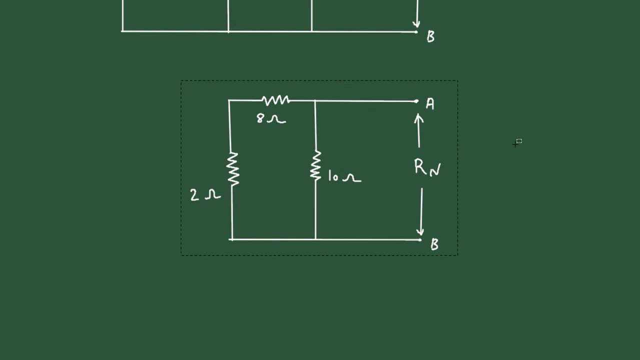 this 8 ohm are connected in series, so it will be 10 ohm. so this will be 10 ohm. now this 10 ohm and this 10 shop are again connected in parallel, so its equivalent will be pi uh ohm it. 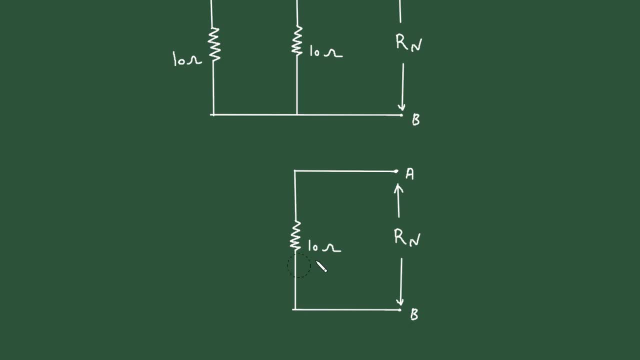 will be of pi uh ohm. now we got the value of R n. R n is equal to pi uh ohm. here we can write: R n is equal to 5 ohm. now we have value of value of Norton's resistance and Norton's current, So we can draw Norton equivalent circuit. 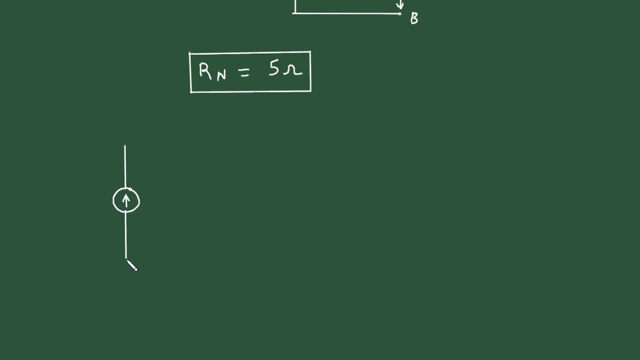 So for Norton equivalent circuit there will be a current source in parallel with Norton's resistance. So this will be IN and this will be RN. RN is equal to 5 Ohm and here IN is equal to. we got the value of IN as 1 Ampere, So this will be: IN is equal to 1 Ampere, So